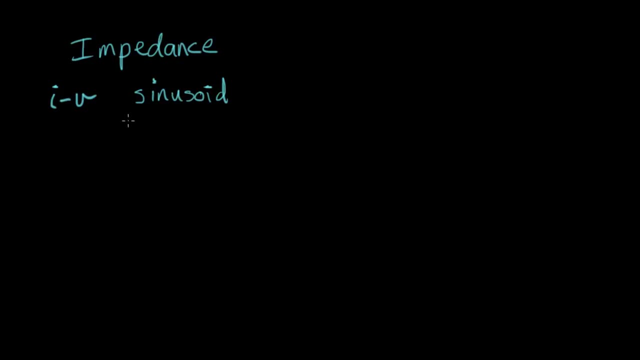 is in the shape of a sinusoid and we're gonna see what that means for the IV equations for our favorite devices. So as we look at our IV equations with sinusoid inputs, we're actually gonna break down sinusoids into complex exponentials. 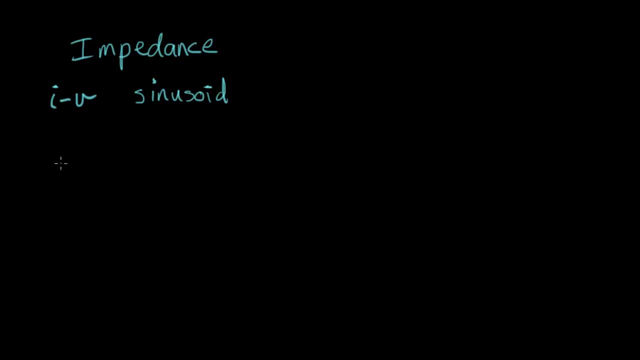 And when we studied sinusoids, we found out that we could disassemble sinusoids into complex exponentials using Euler's equation. So, for example, if we have a cosine wave, if we have a cosine as a function of time, omega t. 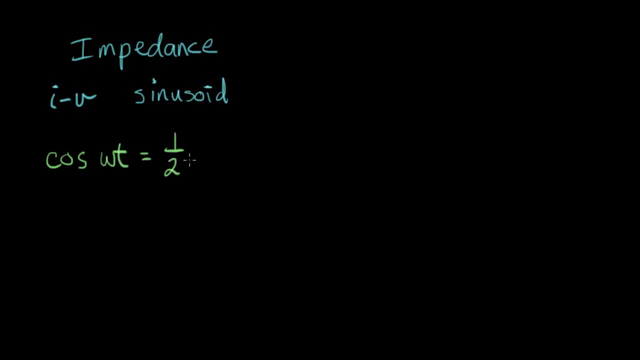 we could express that in terms of complex exponentials like this: one half e to the plus j omega t, plus e to the minus j omega t, Like that. And what I'm gonna do now is I'm gonna say: let's look at what happens when we use this. 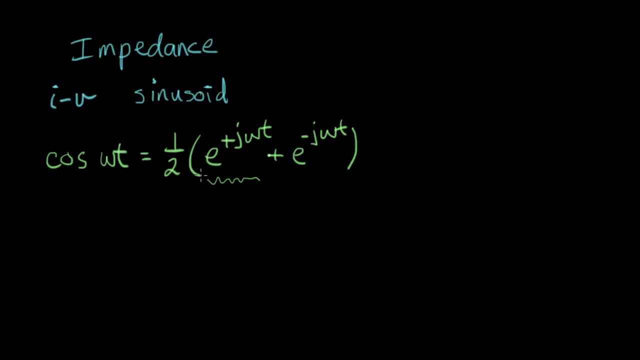 as an input signal. This is not a real input signal, it's an imaginary rotating vector. But if I have two of these, I can reassemble them into a cosine wave. And we like to use these exponentials because they go through the differential equations. 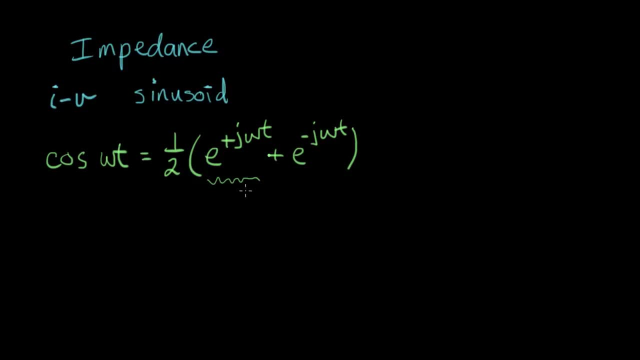 of a circuit really easily. These are the inputs that we know how to solve when we do differential equations. So what I'm gonna do is develop the IV equations for the resistor, inductor and capacitor in terms of this kind of an input. 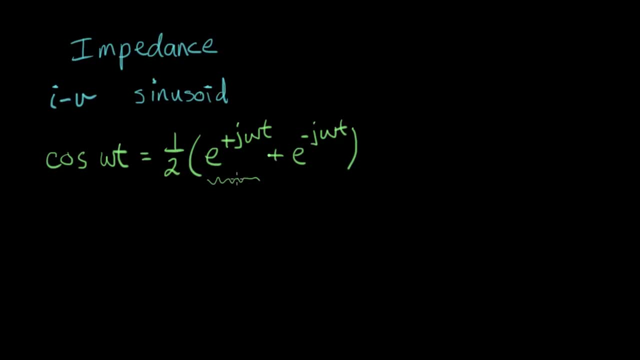 when the voltage or the current looks like this, what do those equations look like? So we're gonna start with. we'll start with the resistor. Here's a resistor And we know from that that just Ohm's Law is: V equals I times R. 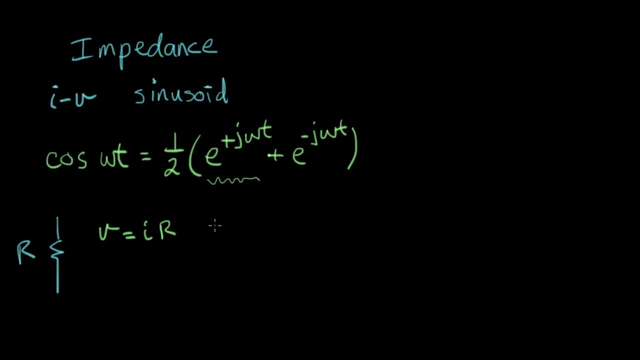 And just for the moment, I'm gonna assume that the current- let's assume that I equals e to the plus j omega t. So if this is I, what is V for a resistor? Well, we just plug I in here and we get V equals R times e to the plus j omega t. 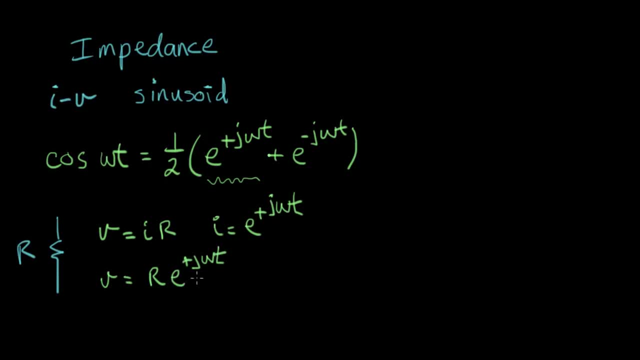 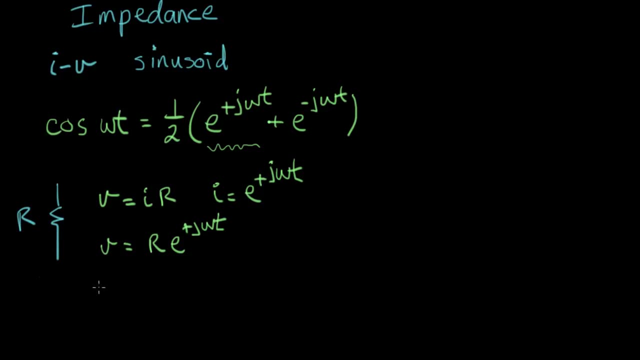 Now I'm gonna do something that looks like it's a little too simple, but it's gonna get interesting soon. I wanna look at the ratio of voltage to current In this situation where we're driving with this complex exponential. So voltage turned out to be R, e to the plus j, omega, t. 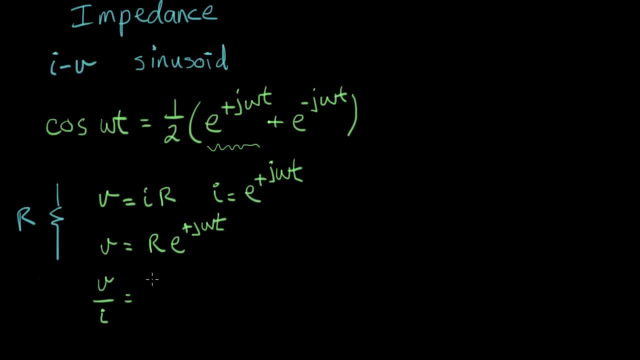 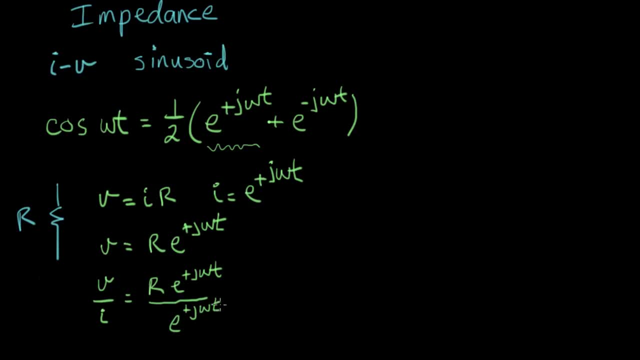 through the resistor of e to the plus j, omega, t. And what is that equal to? Well, these two are the same, so they cancel, And I get. the ratio of voltage to current is R for a resistor. So for a resistor, we just proved. 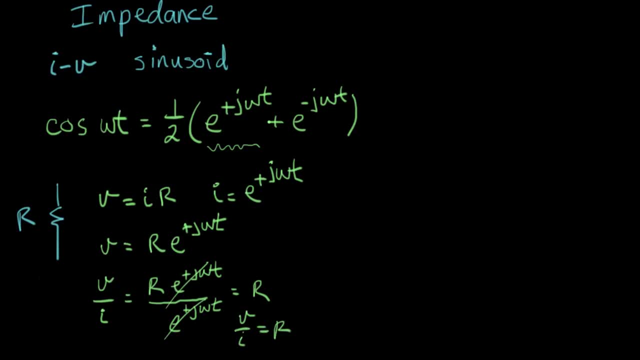 that V over I equals R. So this isn't news. we didn't make a discovery here. this is just Ohm's Law, And for a resistor, the voltage over the current is always equal to the resistance. Alright, this is gonna get more interesting now. 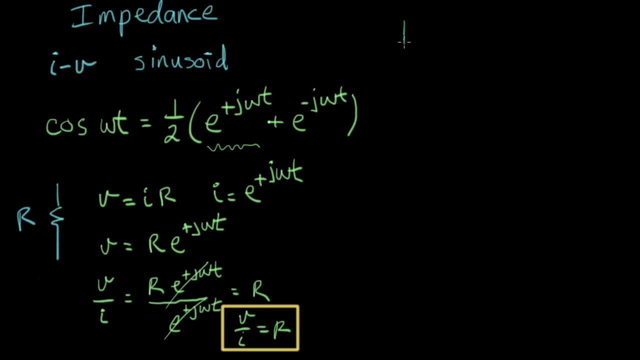 as we go do inductors and capacitors. So let's do an inductor. It has a value of L Henrys, And for an inductor, we know that voltage equals L di dt. And for an inductor, we know that voltage equals L di dt. 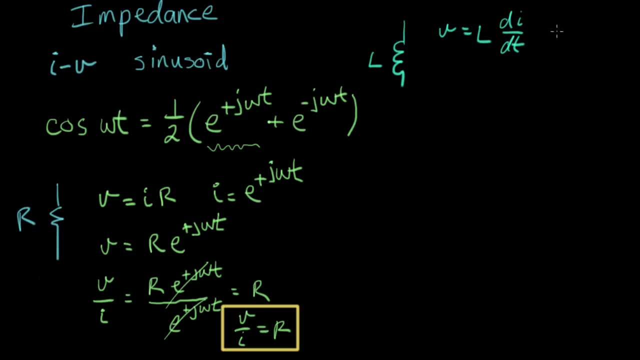 And for an inductor, we know that voltage equals L di dt. Alright, and let's do the same thing again. Let's let I equal e to the plus j omega t. Let's let I equal e to the plus j omega t. 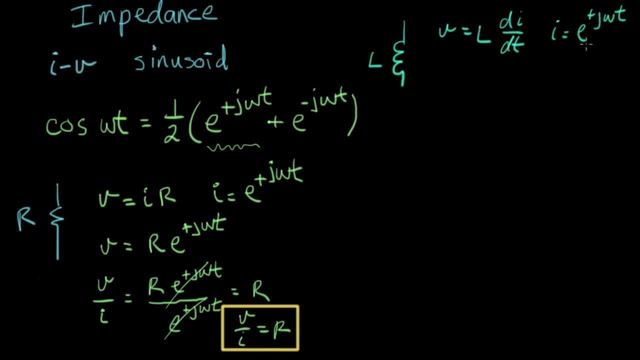 So it's a complex exponential current that we're forcing through our inductor, And let's go ahead and work out what V is. So V equals L times d dt of this value here. So V equals L times d dt of this value here. 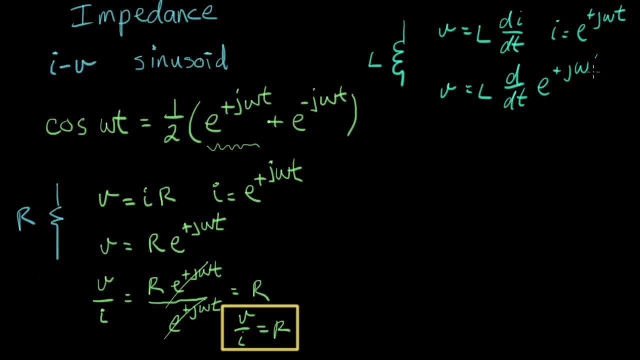 e to the plus j omega t. e to the plus j omega t Or V equals L times d dt of this value. here Now we take the derivative and the j omega term comes down to multiply l, so we get j omega l. 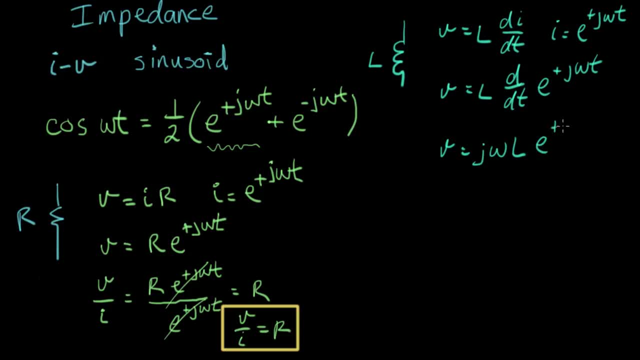 times? what times? the same thing. e to the plus, j, omega, t. This is the beautiful thing about exponentials: They give us back themselves. Alright, now let's do this. Let's take once more: what's the ratio? 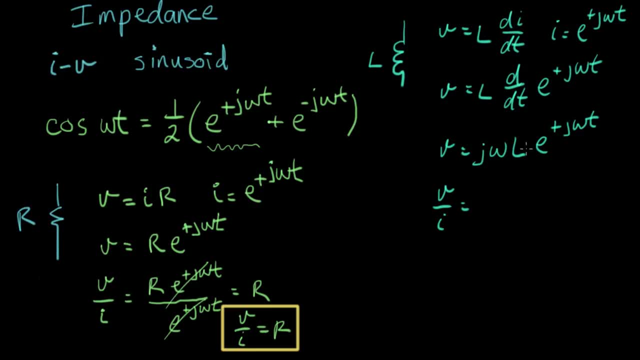 of voltage to current And that equals- here's the voltage j omega l times e to the plus j omega t. And let's divide that by i, which is i is right here. i is e to the plus j omega t. 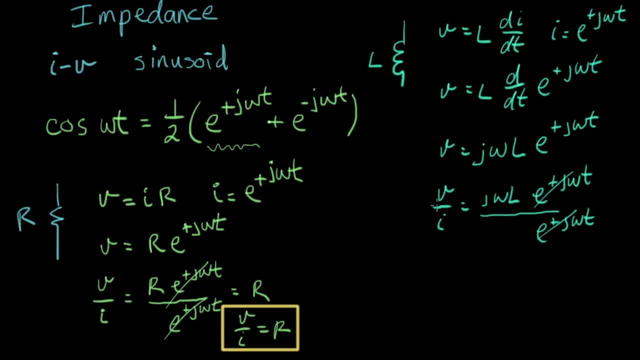 So those cancel and we get v over i equals j, omega, l. So now we have an equation for v over i for an inductor, And this is interesting, This time we have the inductance value which we expected, and there's also this omega. 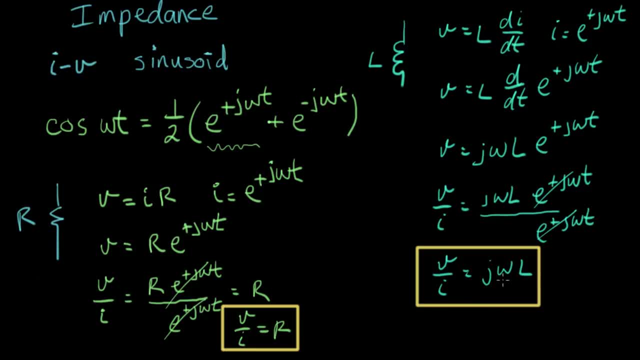 j omega term that comes in. So this tells us: this is frequency, omega is frequency. So this tells us that the ratio of v to i for an inductor is dependent on frequency. Now we'll do the same thing for a capacitor. 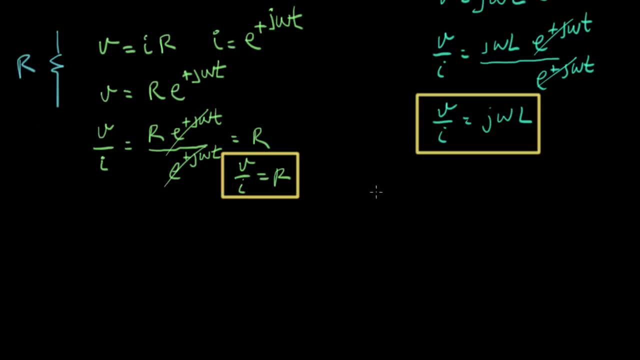 So here's a capacitor And there's it's capacitance value in farads. And for the capacitor, we know that i equals c times dv, dt, And this time let's let v of t, let's let v equal e to the plus j, omega, t. 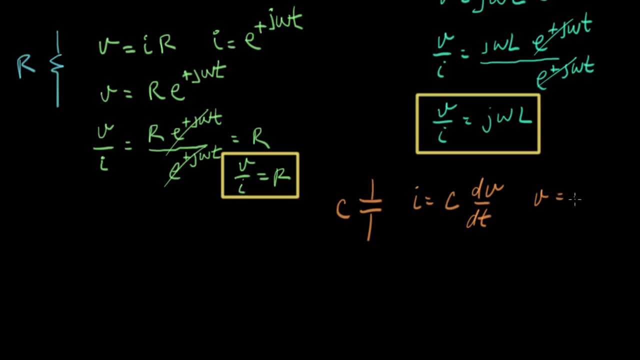 And this time let's let v. let's let v equal e to the plus j, omega, t. So this time we're gonna force a voltage across our capacitor. that is this imaginary, this complex exponential, And that gives us- let's plug that in here. 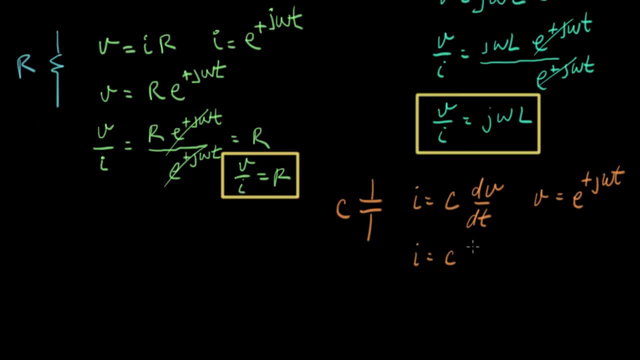 i equals c times d dt of e to the plus j omega t. Now let's take that derivative. i equals, same thing happens. j omega comes down to multiply out in front with c, And we get the same thing over here. So we get j omega c times e to the plus j omega t. 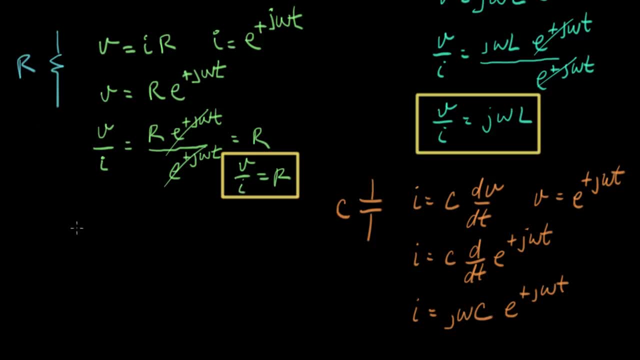 And now we'll ask the same question again that we did before, which is: what is what is v over i for a capacitor? And we can fill this in: v is sitting right here. v is e to the j omega t, e to the plus j omega t. 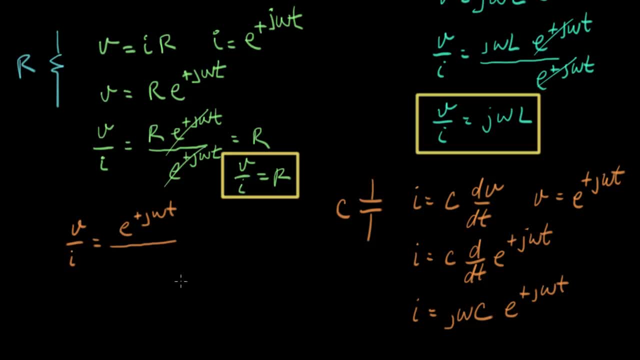 And the current is- we worked that out down here- That's j omega c times e to the plus j omega t, And once again we get this nice cancellation here. This cancels with this And for a capacitor we get v over i. 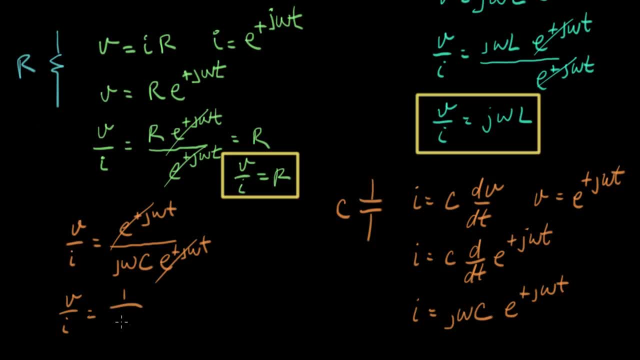 equals equals one over j, omega, c, And we put a box around that one too. So this says that the ratio of voltage to current in a capacitor it depends on the value of the capacitor, of course, And it also depends on frequency. 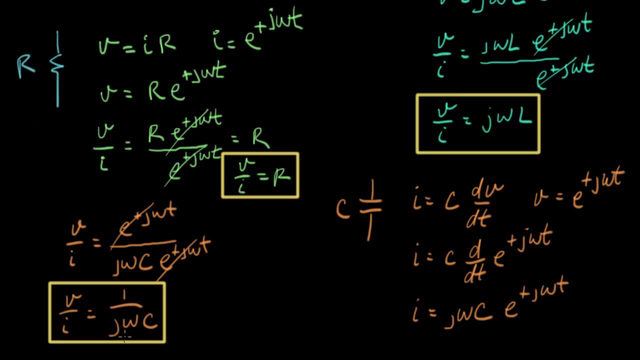 So, just like over with the inductor, we have a frequency term in here. So now we're gonna give this this ratio of voltage to current. in all three cases we're gonna give a special name, and that name is impedance, And the symbol we often use for impedance is a z. 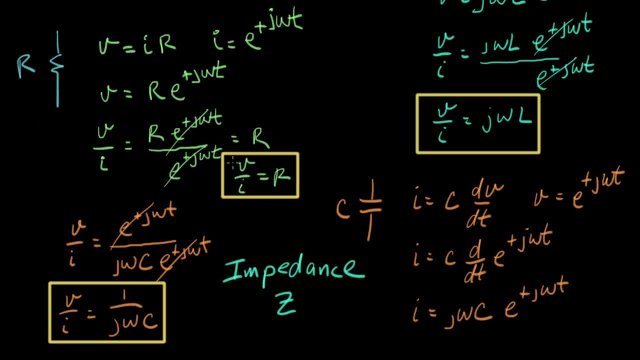 So this word impedance is the general notion of the ratio of voltage to current And we can do that for all three of our passive components. For a resistor, the impedance is its resistance R, So the word impedance is like the word resistance. 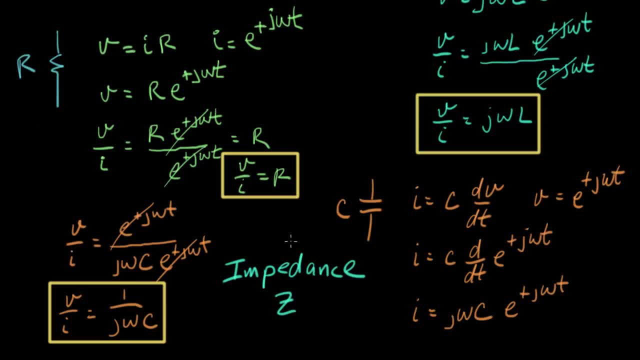 except it's a more general concept. It's the general concept of voltage divided by current. For a resistor, the impedance is the resistance. For an inductor, the impedance v over i is j, omega, l And down here. for a capacitor, 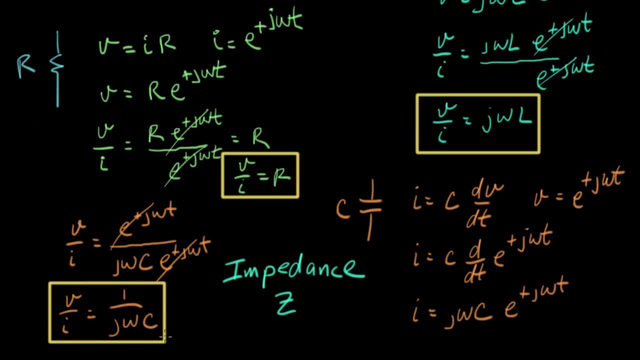 the impedance is one over j, omega, c for a capacitance. So this is where the idea of impedance, this word impedance, this is where it comes from, And the idea includes both the values of the components and the effect that frequency has on the voltage to current ratio.